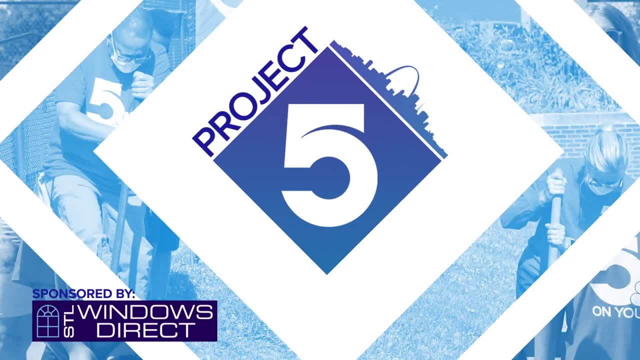 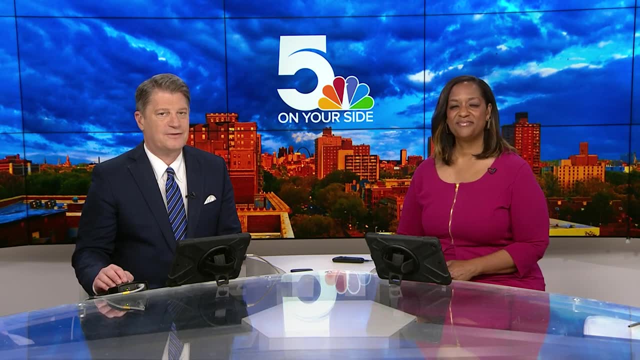 Project 5 is brought to you by STL Windows Direct. Well, today, Project 5, teamed up with an organization called Good Journey and volunteers from STL Windows Direct, helped build a community garden. Now the 18-year-old organization is looking to spread their roots and help grow the next generation of leaders. Ryan Henson shares. 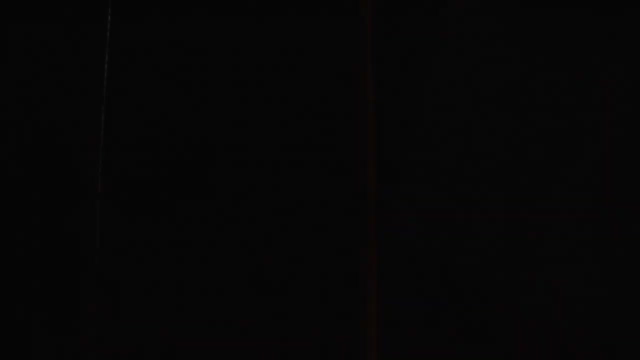 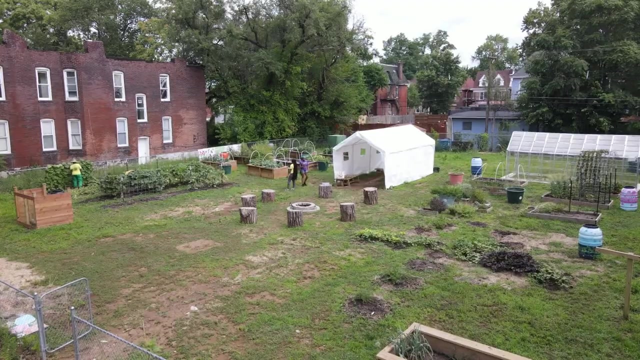 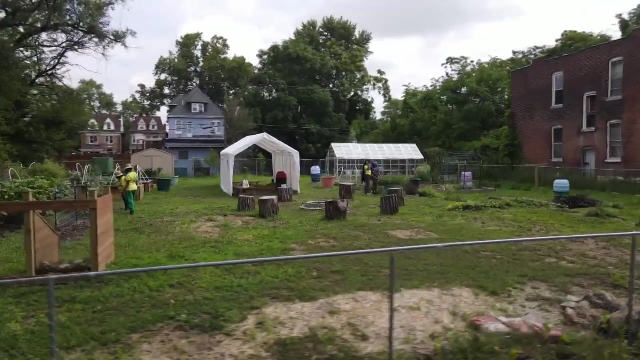 this Project 5 initiative. There's a lot in the Fountain Park neighborhood that's changing the community- Bustani Ya Upenda, which means in Kiswahili, garden of love, And we have seen growth in our young people as far as their leadership skills, ability to get things done. 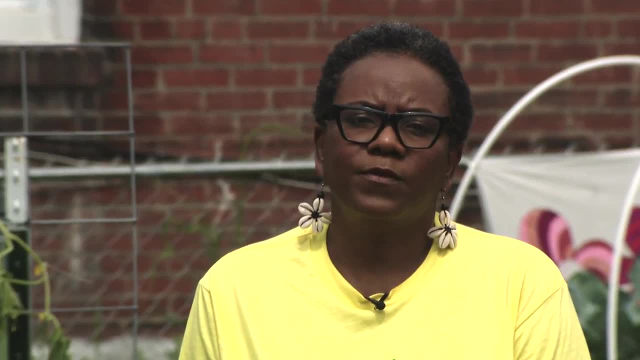 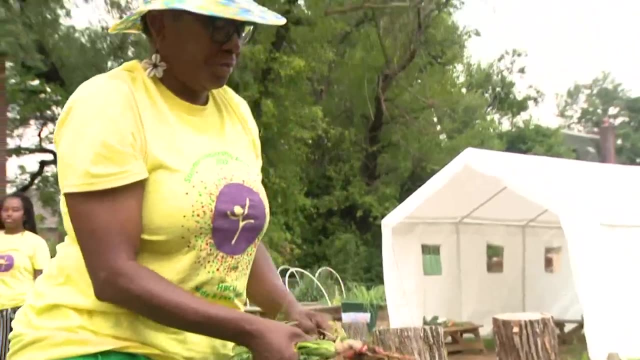 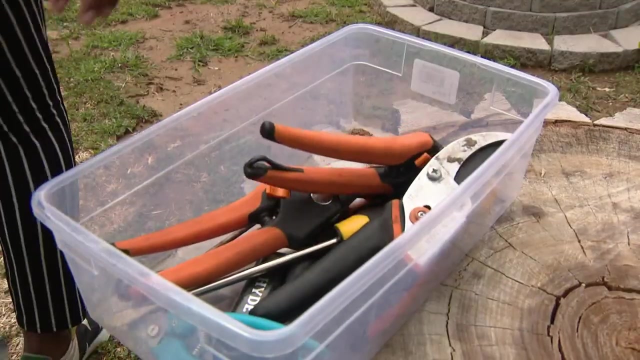 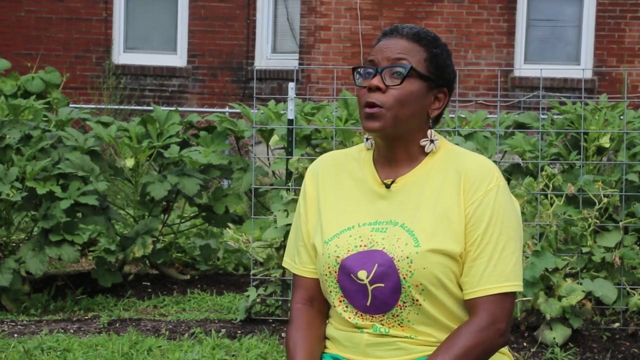 to take lead on on certain things. We've seen the growth as far as healthy, healthier eating. The executive director of Good Journey says the students planted the seeds to create a community garden in 2020 and it's been thriving ever since To see young people as assets and experts in our community. to make sure that they have the space. 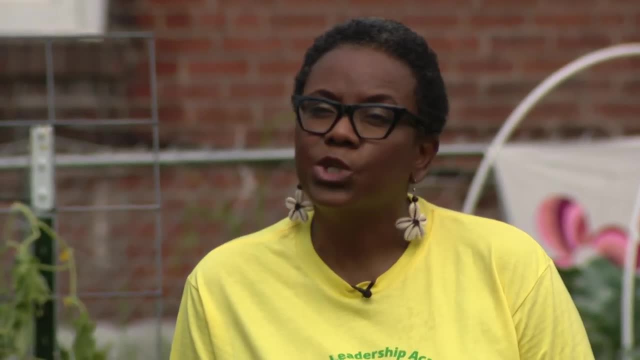 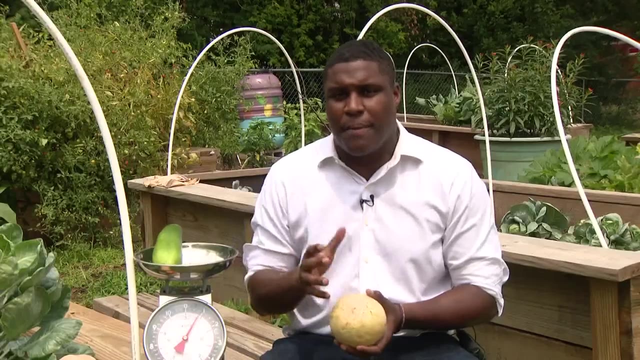 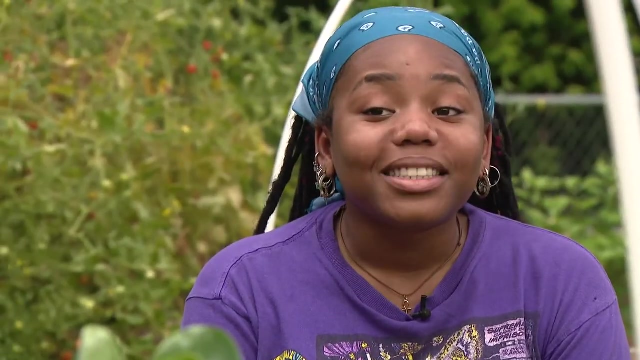 and opportunity to work on issues and community that are important to them, like this garden. Mama Dionne says this garden really tips to scale to make sure younger generations have the proper leadership skills to be successful in life. We recently got some strawberries. We got to taste the strawberry. 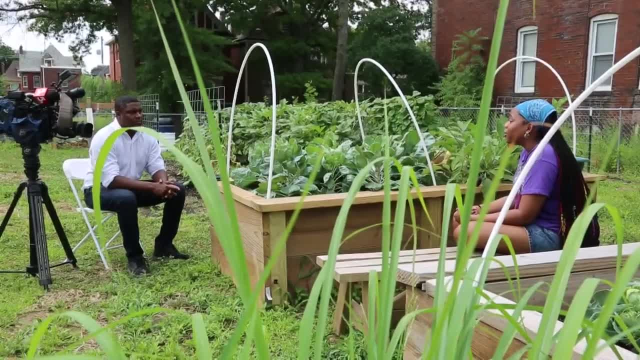 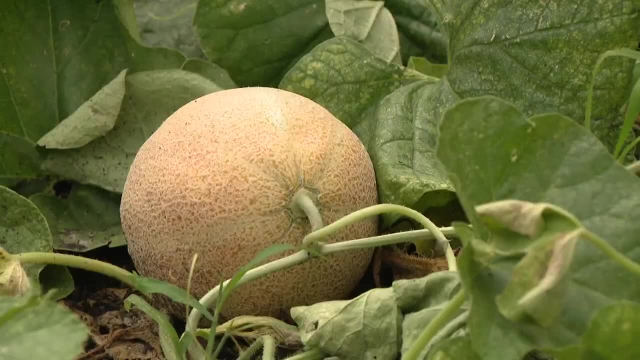 It was so good. Heaven Uhuru is an aspiring chef. She says learning new foods and the hard work of what it actually takes to get an idea off the ground is a valuable life lesson. The ground was absolutely terrible, unworkable, but we cleaned it up. 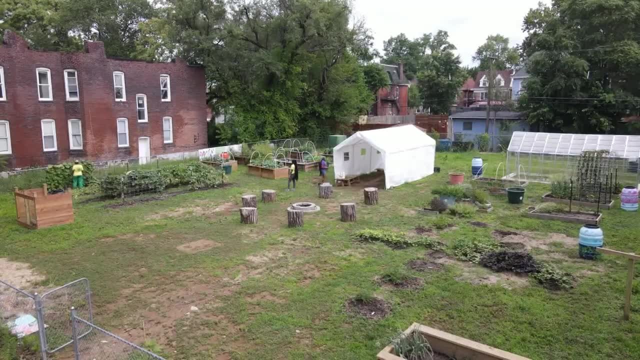 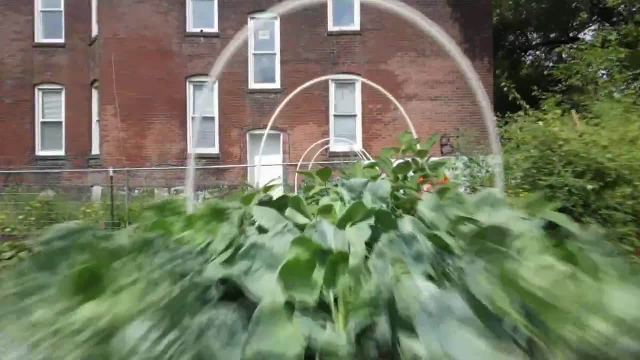 We got all the brick and all the trash out and we were like, yeah, now we have a garden. So this is our herb section. Over there we have some okra, some cantaloupe. If it grows, gardener Bisa Adaro is going to pick it. 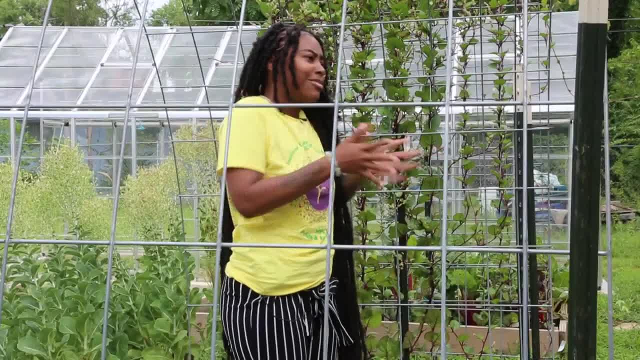 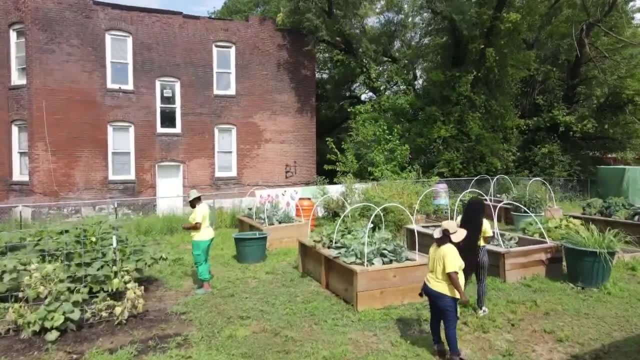 I live around the corner, so if I ever wanted to come over here and grab a tomato or two- maybe some fried green tomatoes or anything. A new, healthier lifestyle Bisa's trying to get more teens and kids into. She's been involved with Good Journey for 10-plus years.